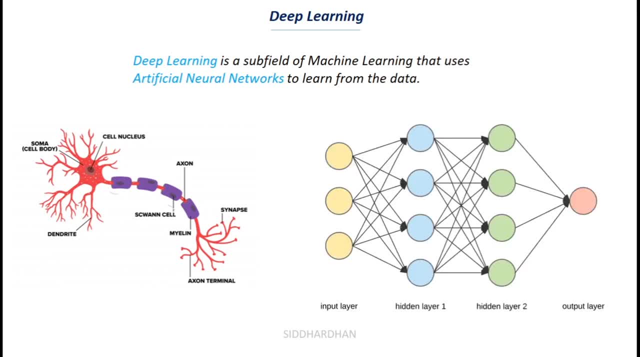 you can see here, this is the diagrammatic representation of the artificial neural network code. so basically, what happens is we have individual neurons connected to each other, which forms the neural network. okay, so each neuron has a mathematical function assigned to it. so this neural network code is a mathematical function assigned to it. so this neural 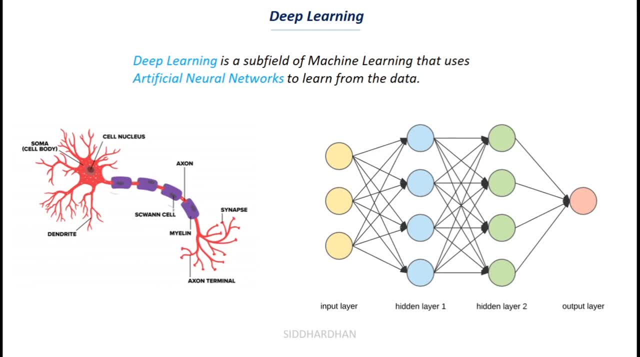 neuron processes. the data say, for example: we want to, you know, recognize what is the image represents. so we want to basically do an image recognition task. so we feed the image to this neural network and in the input layer this image will be splitted into it its respective pixels. so there will be a lot. 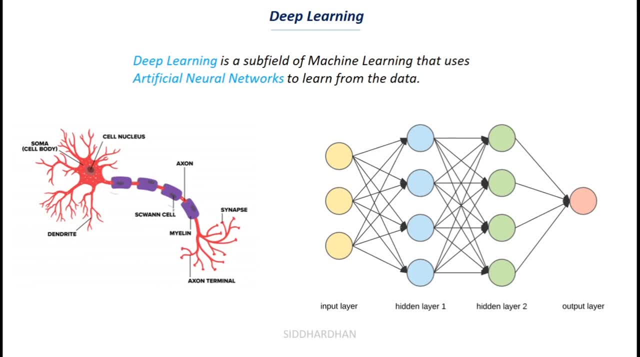 of pixels and each of these pixels will be given to several neurons and in the input layer this information, this pixel value, will be processed and it will be transferred to the hidden layer and then again there will be some process, there will be some processing happening in the hidden layer and then it will be. 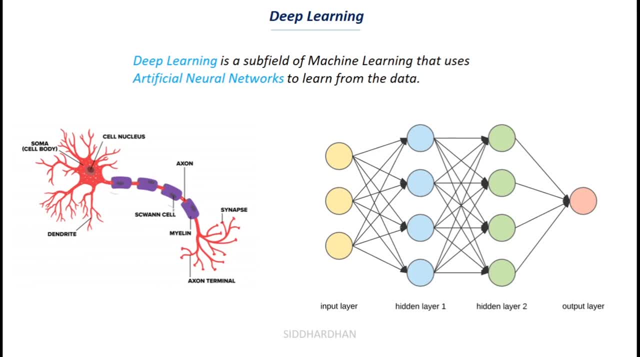 transferred to the output layer where the image is predicted. okay, so this is how the neural network works. so, as I told, there are three main layers in the neural networks. so first one is the input layer, then is the hidden layers and finally we have output layer. okay, so there can be any number of hidden layers. 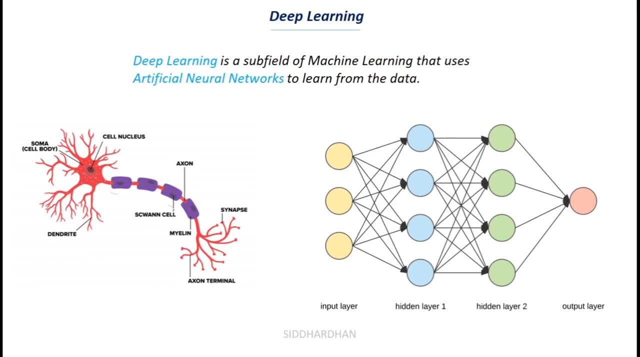 in a neural network, depending on the task we are doing. okay, so each neuron has a mathematical function. so, as I have told you, and this process information, and each neuron in the input layer is connected to each neuron in the hidden layer. okay, and this is how the information is passed and the 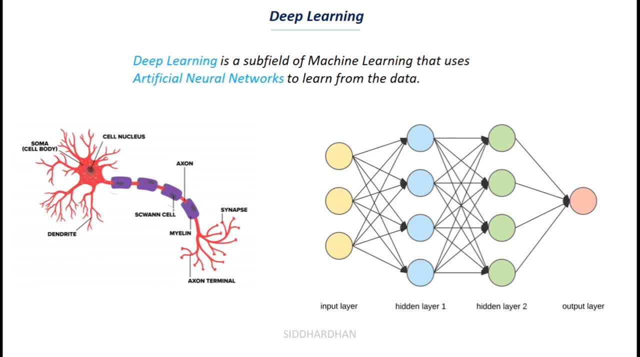 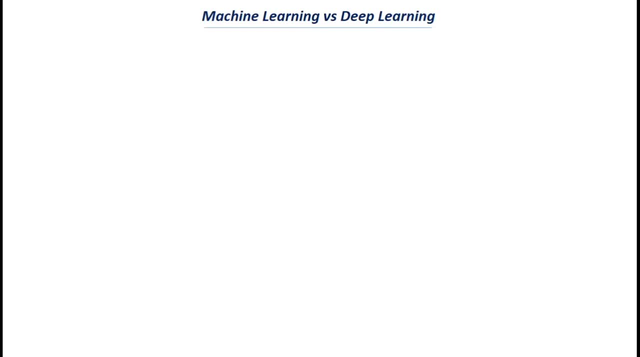 respective prediction is made. okay, so this is all about artificial neural networks. now let's try to understand what is the difference, the main difference between machine learning algorithms and deep learning? okay, so rather than difference, it is. you know, deep leaning is one main advantage over machine learning, so that your difference is feature extraction. okay, so what is meant? 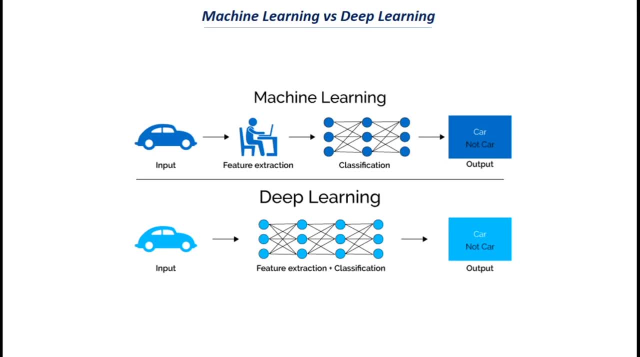 by this feed extraction. let's say that we want a machine learning model to predict whether a image represents a car. okay, so when you are giving it to a machine learning model, we need to tell the model that these features are important for a car. okay, for example, if it is a car, it should have four wheels and it should. 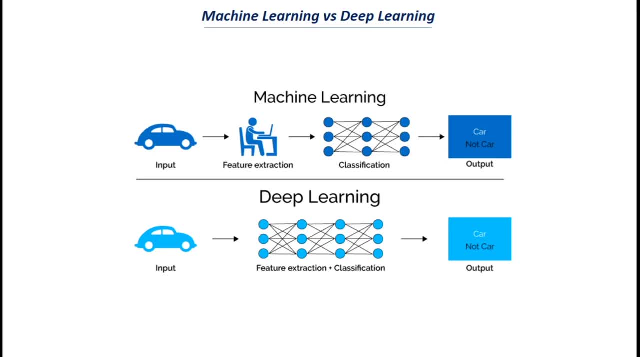 have a shape like this and all that right. so we need to give those features to our machine learning model. we have to manually tell them that these features are important. but we don't need to do that in the case of deep learning because the neural networks are so much powerful than any machine learning. 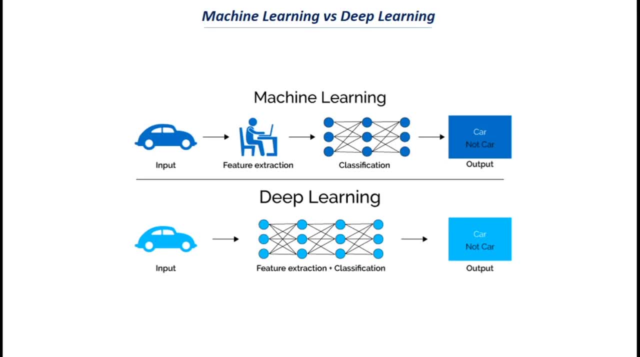 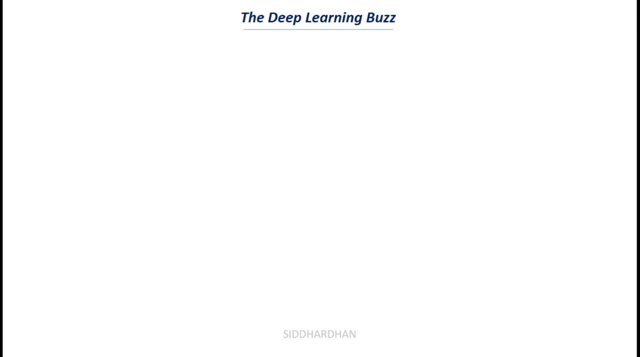 algorithms, they can determine those feature by themselves. okay, so that is the main advantage of deep learning or machine learning, where we don't need to extract the feature manually. okay, now let's try to understand the events that made deep learning so much popular. okay, so there is a famous deep learning. 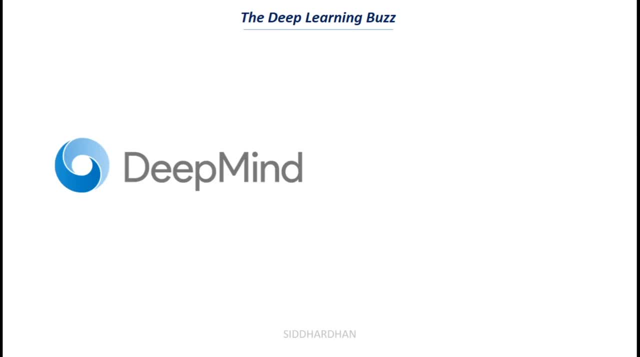 company called as deep mind, so it is based in a United Kingdom, so it was started around the 2000s, so deep learning was there, you know, from that point of time and even before that. so what happened is, in 2014, Google acquired this company, so deep mind. 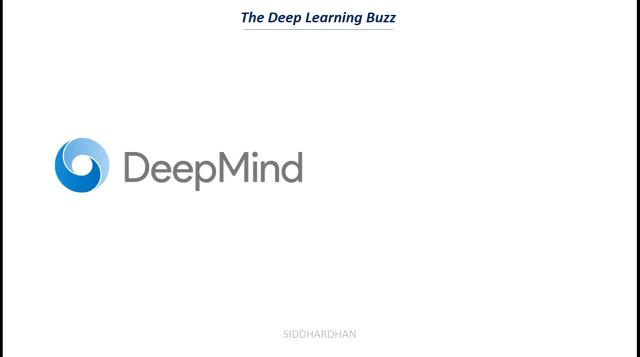 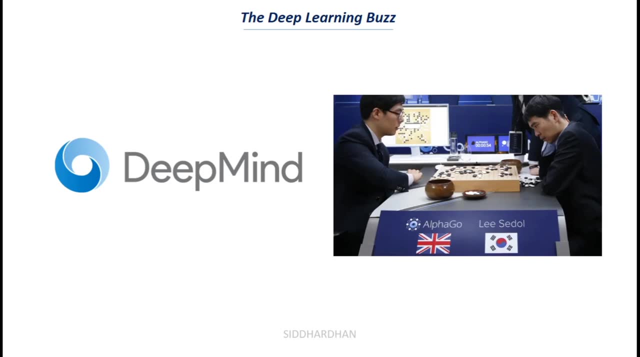 basically made game playing artificial intelligence system. okay, so there is this famous game called as go. so this go, this board game like chess, but it is so much complicated and so much, you know, deeper than chess, because in chess there is limited number of moves one can make, but the possibilities in go is so much. 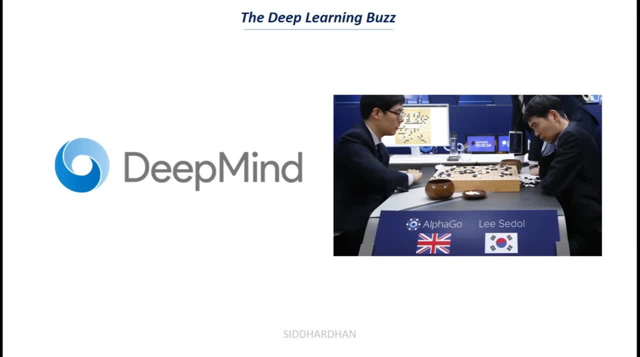 more, so there are several moves one can make based on the configuration of the game. okay, so in 2016 they made a machine learning- sorry, our deep learning system- that can play this go game and they challenged the world champion, Lee Sedol. so he is 18 time world champion and they challenged him for a five match. 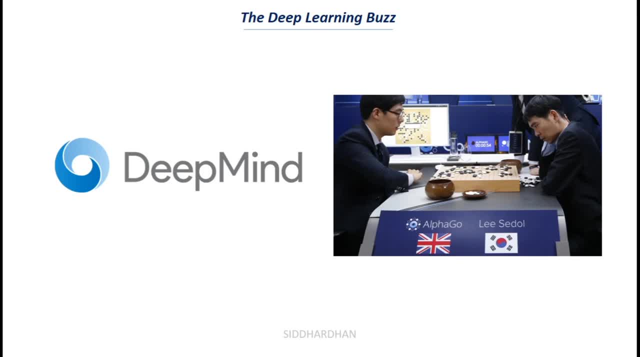 tournament. okay, so that game playing system was made based on deep learning. okay, so they have been developing this over, you know, five or six years and they challenged him and what happened is in the tournament of five games. so alpha go, which is the system deep mind build, has beat Lee Sedol, for four is to one. 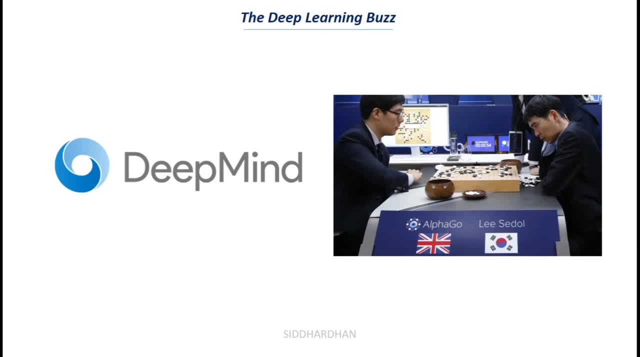 okay, so it has won four matches and Lee Sedol won one matches, and that is where people started to look at deep learning and realize that deep learning is so much powerful than any other algorithms in machine learning. okay, so after that, several researchers were made and several modifications have been done to 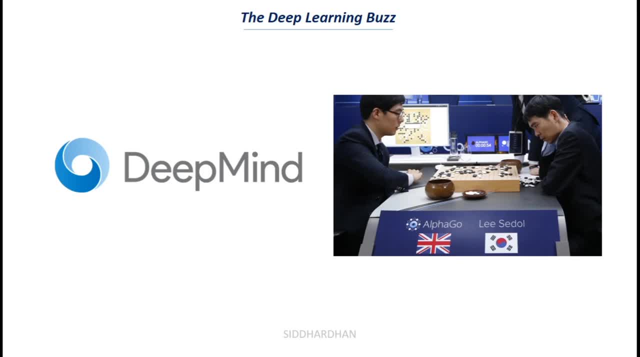 the neural networks in several different types of neural networks have been, you know, invented, as you know, this is the basic technology of deep learning in. you know, invented, as you know, this is the basic technology of deep learning, So that it is accessible, especially for people who know deep learning. so that's. 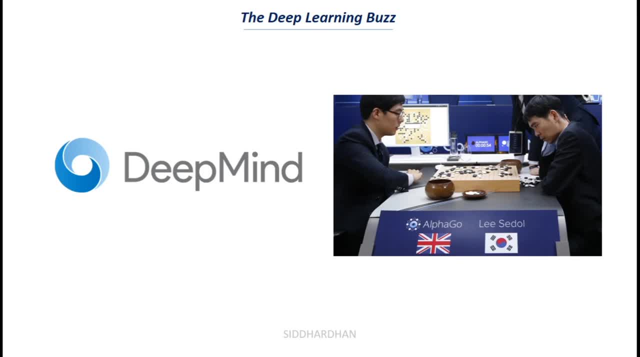 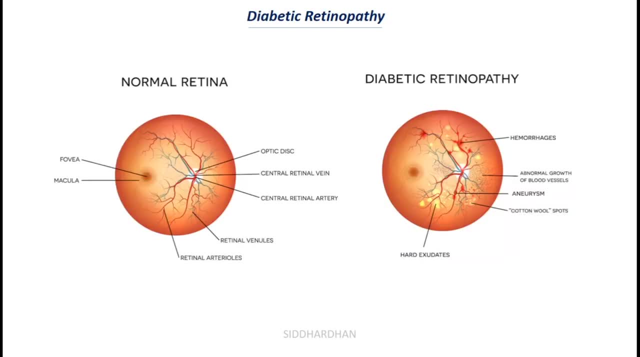 after that. so this is the point from which deep learning got so much you know, popular and it was used in several kinds of fields after that. okay, let's try to understand one such example for this. so diabetic retinopathy. so diabetic retinopathy is a condition where a patient may lose his eyesight. 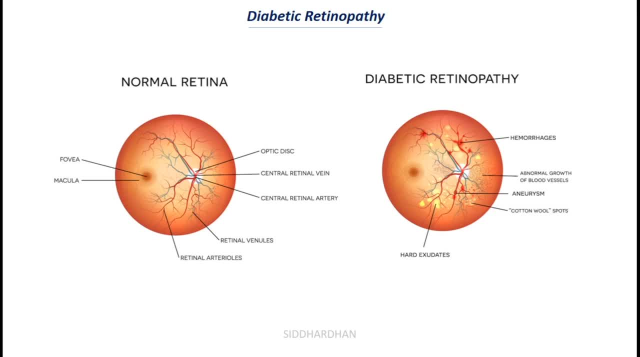 lose his vision due to diabetes mellitus. okay, so this deep mind developed a system based on deep learning that can determine whether a person has diabetic retinopathy from the eye scans. okay, so how this is basically made is: the deep learning model will be trained with several normal eye. 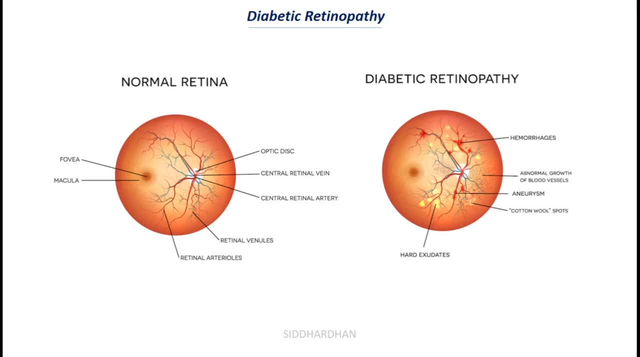 images which does not have any disease, and the model will be again trained with several images. which has diabetic retinopathy? okay, so once it trained, when a new image is fed to this model, it can predict whether the person has diabetic retinopathy or not. so the interesting thing, 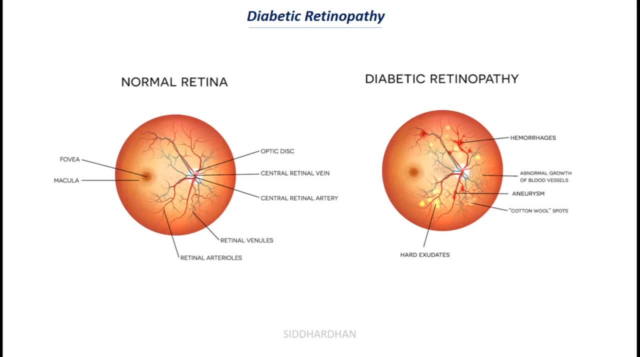 that happened here is it doesn't only you know the person has diabetic retinopathy or not. so the interesting thing that happened here is predicted whether the person has diabetic retinopathy or not. it also predicted the gender of the patient, whether you know the image of the is of a male or a female. it also predicted 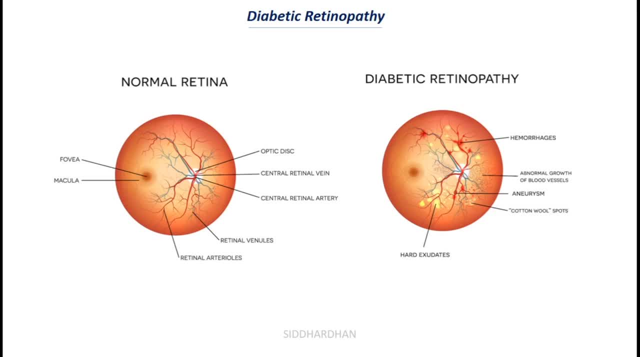 whether they have some some other medical conditions or not. so this is one of the fascinating thing that happened, where the deep learning also predicted several other things, rather than only the patient has diabetic retinopathy or not? okay, so these events led to the boom of deep learning. after that, it was used in several other 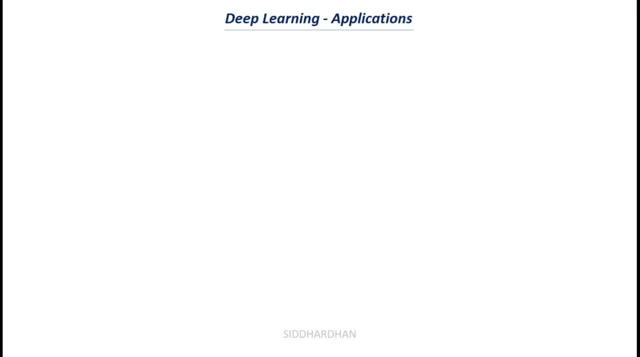 other features. now let's discuss about some of the important applications of deep learning. first one is health care. okay, so, with the example which we have seen now is an example of health care application. so, apart from this, deep learning is used in several diagnostic departments. where it is used, 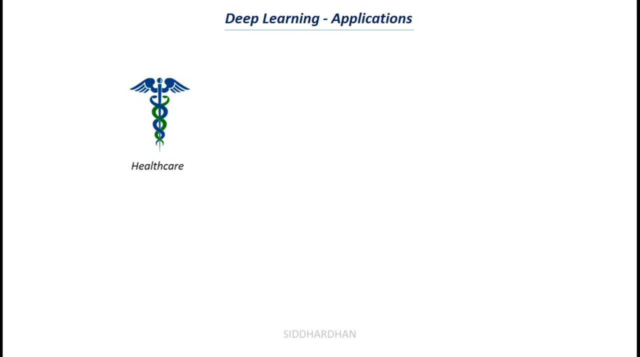 to predict whether a person has a specific, specific disease or not, based on their scans, images and other data. so another example where deep learning used is the field of autonomous cars. so autonomous cars, like Tesla, doesn't need a much more much driver input to drive the car right, so they can drive the car by themselves and it is. 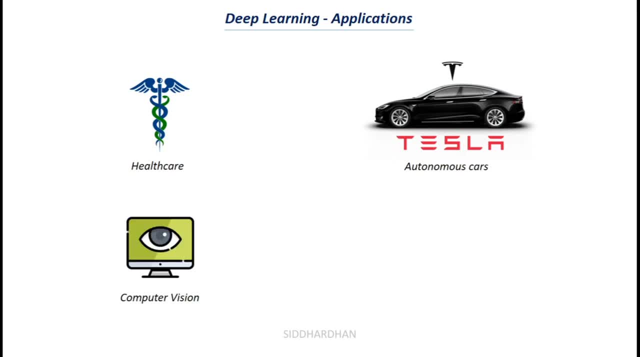 powered by deep learning models. then we have computer vision. so computer vision is one of the important application of deep learning. so it is based on image processing techniques, where the neural network is trained with several images. so one such example is face recognition system in our phones. so it is based on computer vision. then there is natural language processing.